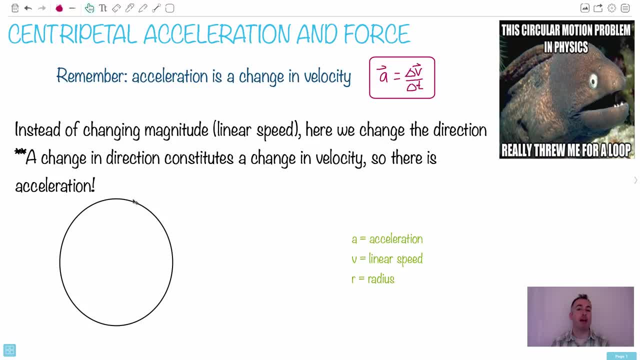 go in a nice straight line. Think about this: if you're only allowed to give it short little pushes, you know, you can sort of apply a little impulse. we would say, right, that makes it change its momentum. So let's say, you just apply a little like a little push, a little force, you kind of boom, you just 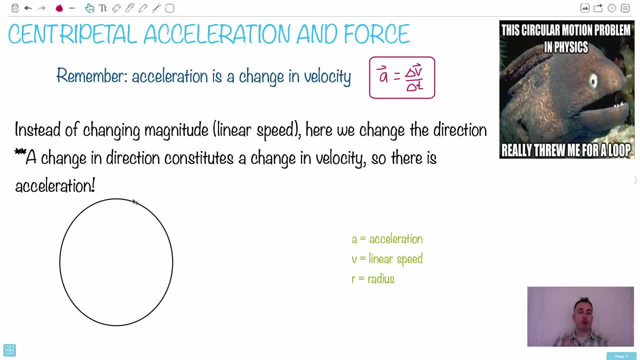 sort of hit it lightly. If you wanted that ball to go in a circle, how would you do it? Imagine this: this ball is going straight up. let's say you could give a little tap that way to left, and then maybe another tap that way, and then another tap that way, another tap. You can see it's going to. 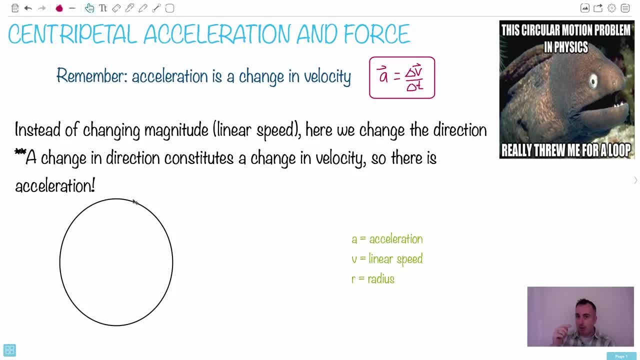 go in a circle. You can see each way you tap it. Imagine which way you have to hit it. Think about which way you'd have to hit it. You'd have to hit it. you know this way. then it would be going that way. then you'd have to hit it that way and that way. Look at which way your force is, Isn't your? 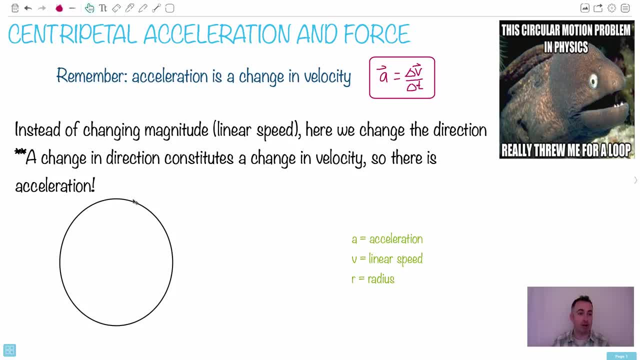 force always acting towards the center. That's why we call it centripetal. Centri means center seeking. That's what this means. This is center all right, the American style with the er like this: Center seeking. That's what center seeking is. 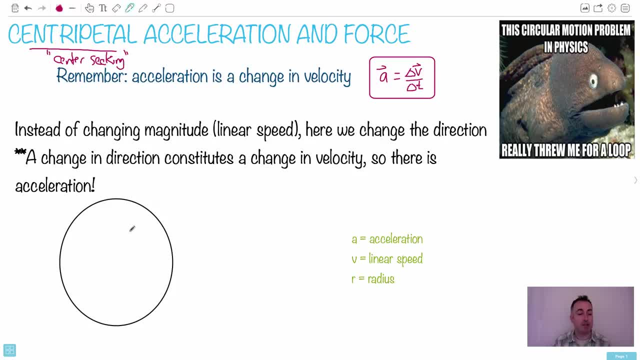 Center seeking. That's what center centripetal means. This is because as you go around in a circle, there's technically a center force. If there's a center sort of forcing- sorry, directed force, do you see there's also a center acceleration. I mean, that's better to put the acceleration. So you're gonna. 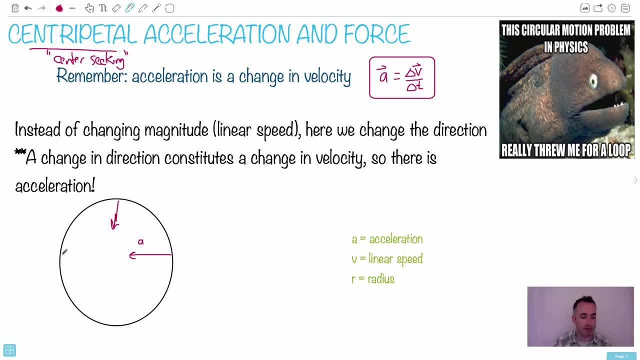 have an acceleration inwards. It doesn't seem like it, but you're actually going to have a center pointing acceleration here. Okay, and that's because, again, you've changed your velocity, So even though your value of your speed stayed the same, you know. so imagine you have just 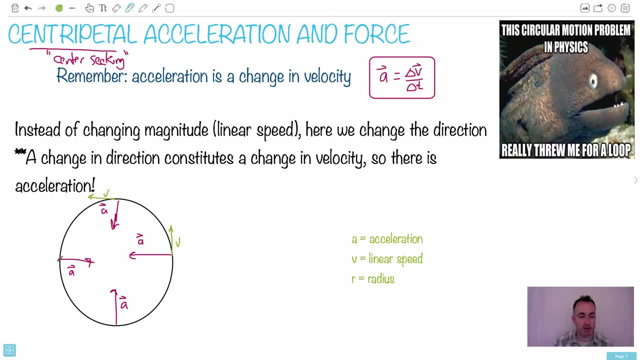 you know V here. So the actual length of that vector stayed the same at all points in this thing. that here's motion, That's assuming you're going to the right, like like this counterclockwise, You could say that well, the value of the speed doesn't change. Maybe you're going like I don't know, eight. 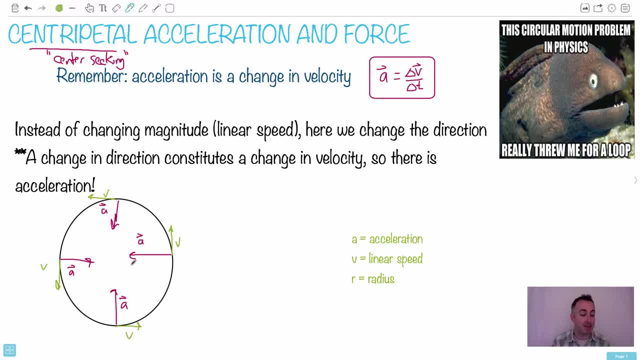 meters per second all the time, but your direction is changing. because of that, you have an acceleration and the good news is, excuse me, you don't have to change the speed. You don't have to change the speed. to memorize this, You have an equation for the centripetal. See the center seeking: 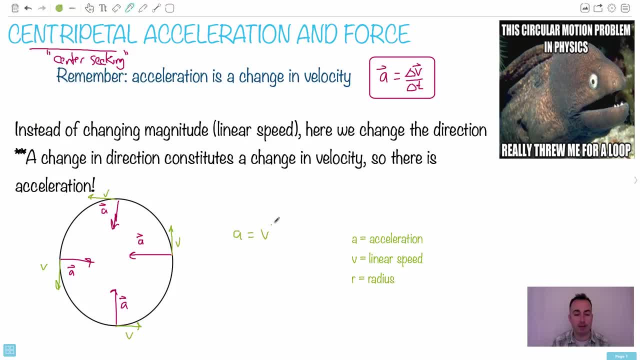 acceleration. It goes like this: A equals V squared over R, So again, don't have to memorize it. There it is. What does this do for you? I like to label it with a little C, C for centripetal. It's technically a vector, but we'll leave it like that. So acceleration is in meters per second. 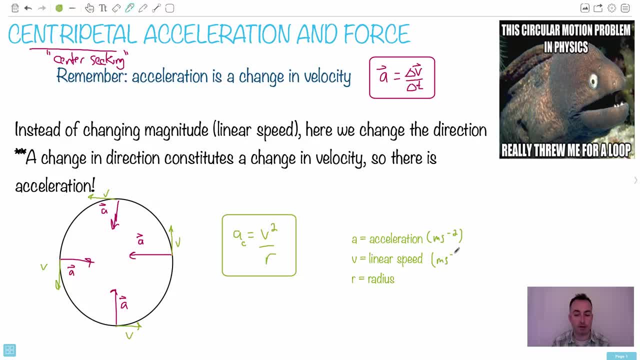 squared. Linear speed, I hope you see, is in meters per second and radius is in meters. So hopefully you'll see that if you do linear speed, which is meters per second, you square it, you get meters squared per second squared and then you have meters on the bottom, So this becomes meters. 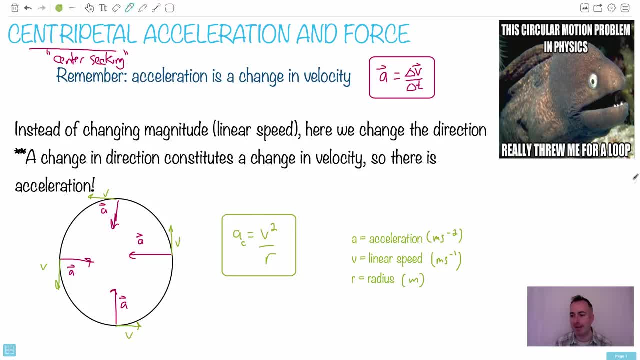 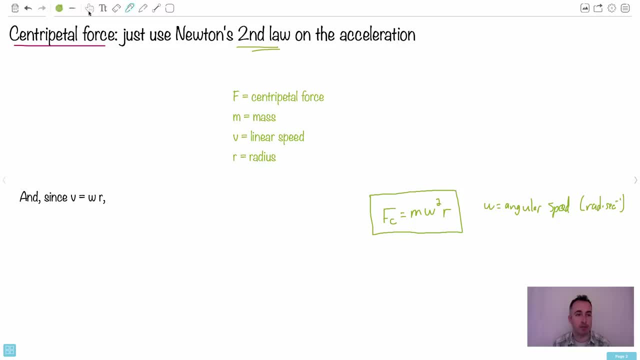 per second squared. So the units work out. Let's look at centripetal force. To do the force, you just use Newton's second law on the acceleration And remember the acceleration was. just remember acceleration is V squared over R. Well, isn't Newton's second law. I mean one of the formulations. 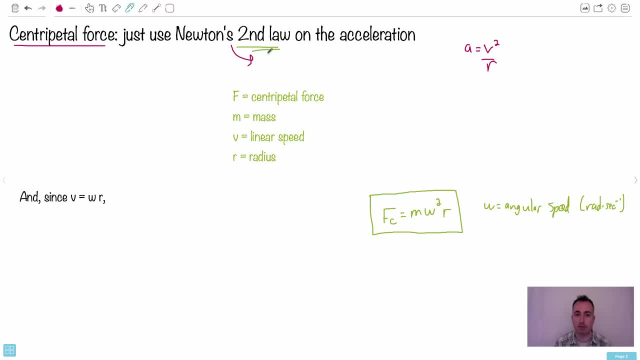 of course it's with a change in momentum. So it's a change in momentum, So it's a change in momentum. You know, you could say F is it's related to a change in momentum. But in this case let's use the other form, probably the more common one, which is F equals MA. That means all you have to do to 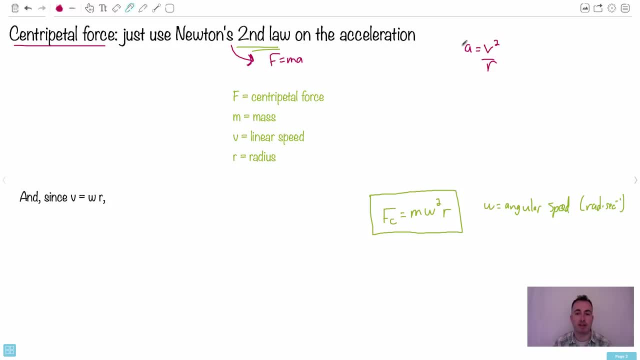 get the force you just multiply the acceleration times the mass. So in this case, right here then, does that make sense? then I would say: then, fine, F equals MA. So that means I would multiply mass times acceleration, which would be mass times V squared over R. That's why I end up with very 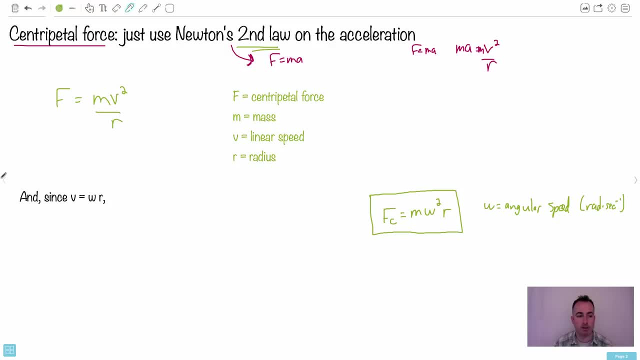 good results. So you just take your acceleration. you had before V squared over R and you just multiply it by an M. That's not that brain busting, right? I hope not. So there we go. There's our equation. And again, just to make sure we know, centripetal force, This is the force acting towards. 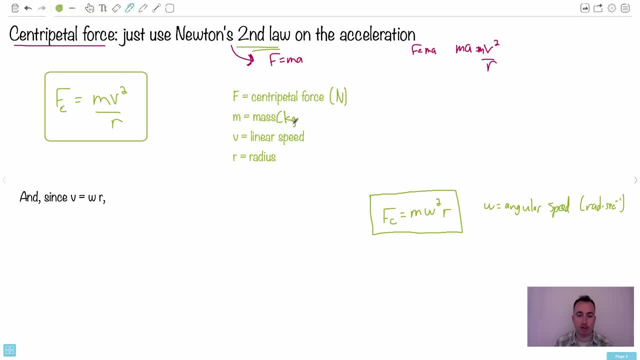 the center. It's measured in newtons, Mass is in kilograms, Speed is in meters per second And the radius is in meters. Just so we have all the right units. And what I like is that when you're looking at, the equation is this: You can see this because from before we have: V equals omega R. In other words, we 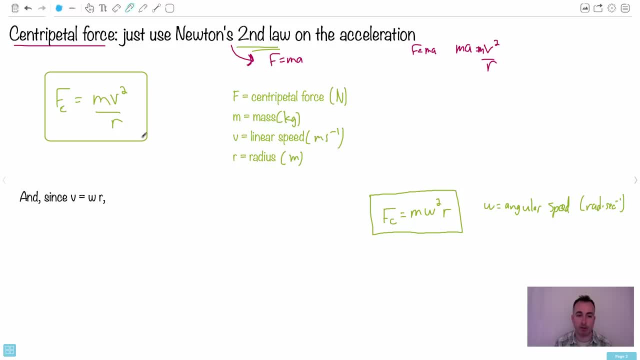 have. the angular speed is related to the linear speed. Here we've been talking about linear speed right In meters per second. So because of that, look, we can replace. We can say F equals M. Instead of V squared we put in omega R squared. Do you see that This is? this is V according to this. So 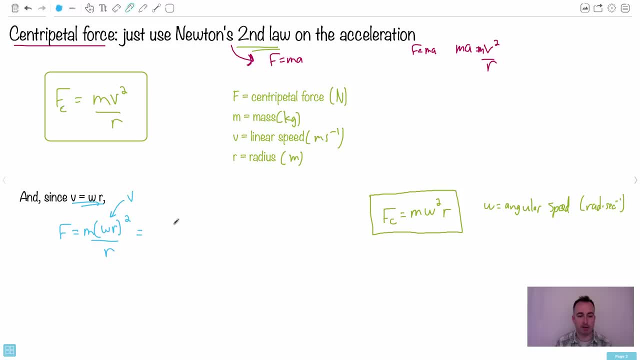 because of that, I have M and then V squared, So that's omega R. So therefore I have F equals. let's see it leads to F equals M. And look at this: I have omega squared, R squared over R. And if I have R, 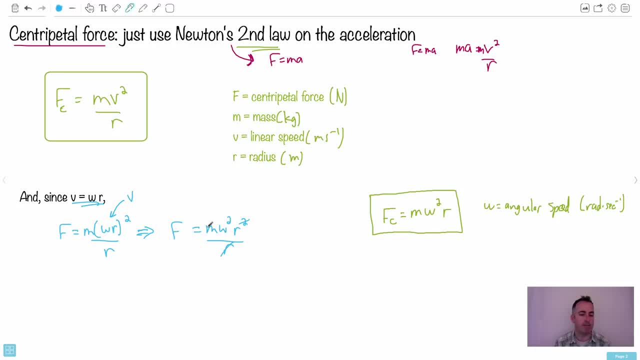 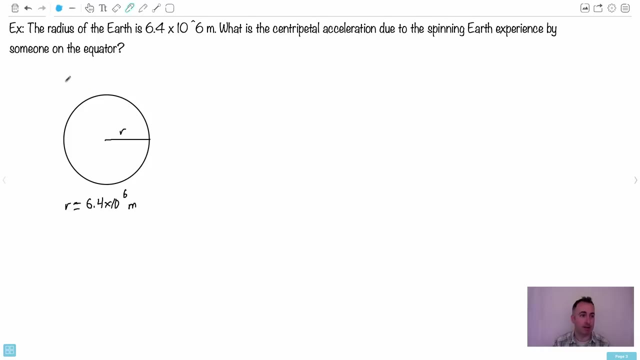 squared divided by R. that one cancels out that one, So I'm left with just: F equals M, omega squared R. Hey, look, And remember that omega is your angular speed, which is in radians per second. So do you see, actually it's not that that bad. Now I have an example for you. Maybe that's a good one to have. 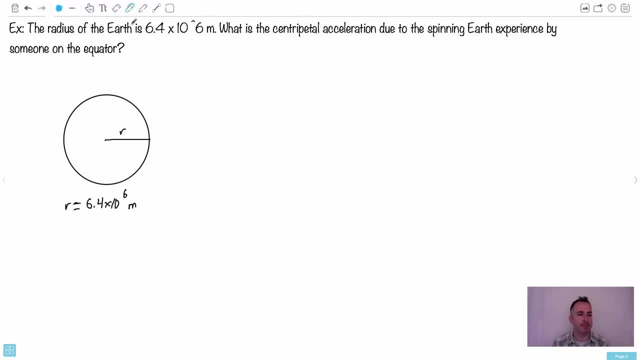 So we're looking at here, we have a radian And we have the radius of the earth, So it's 6.4 times 10 to 10 to the 6 meters. Okay, so that's important, So maybe I'll just write it down. So R equals this. I just didn't really like the notation. 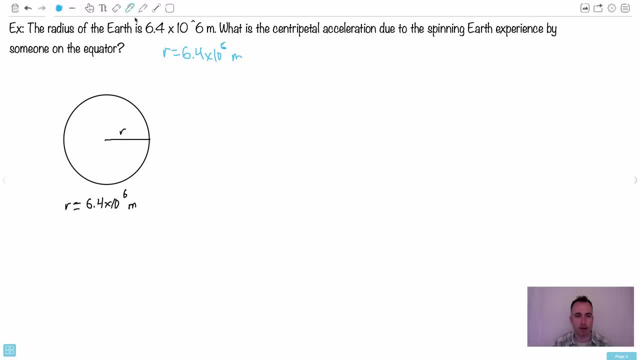 of the font I'm using. So this is more clear, right? Maybe not. Actually, my 6 looks terrible. There we go, I'll make it better. 6 meters: What's a centripetal acceleration? Do the spinning earth experienced? Oops, I should have really made it experienced. 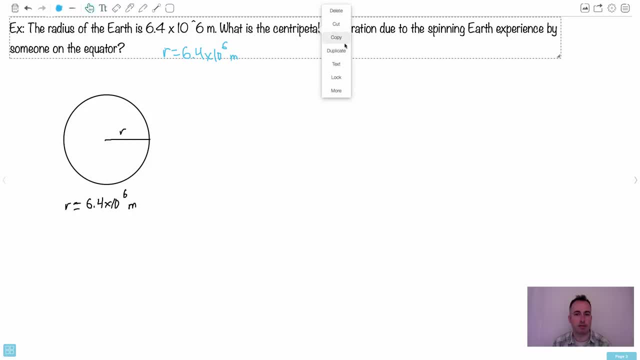 Didn't I? I'll just fix that right now. Hold on a second here. I just don't want to be too many spelling mistakes. at least There we go. So what I want to do here, Here I need to sort of figure out. 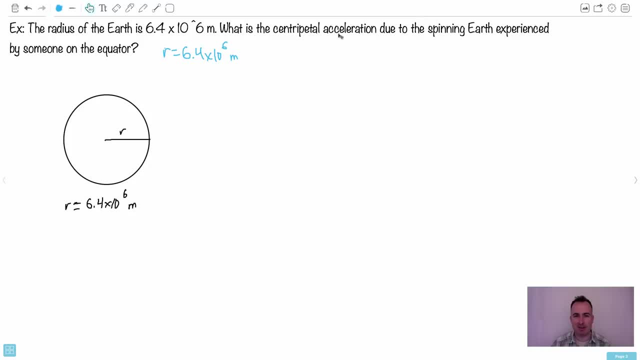 yeah, kind of what to do. So if I have a centripetal acceleration, I can actually figure this out. I can find the acceleration itself. We have an equation for it, don't we? We have the equation right here: Acceleration is V squared over R, So we're going to put that in. So we're going to have to find. 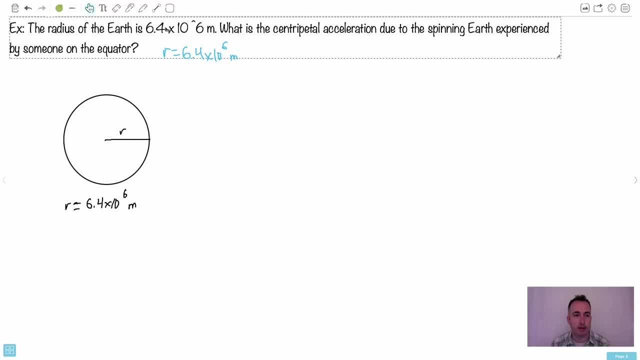 the acceleration, then I'll use this equation here: Acceleration is just V squared over R. Now I know R, which is really good, but I don't know V, Do I? But it turns out I kind of do. You can kind of figure it out, because you can say that V is a distance over time. Remember, V is your. 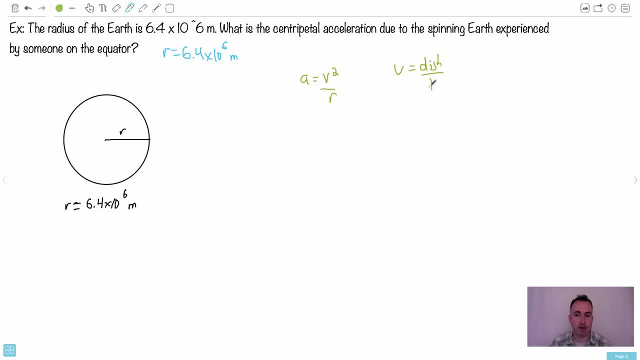 linear speed. So because of that, V is your distance over time. And remember, if you go all the way around in a circle, what you're going to get is a distance over time. So if you go all the way around in a circle and your distance travelled, it's a circumference of a circle which is 2 times. 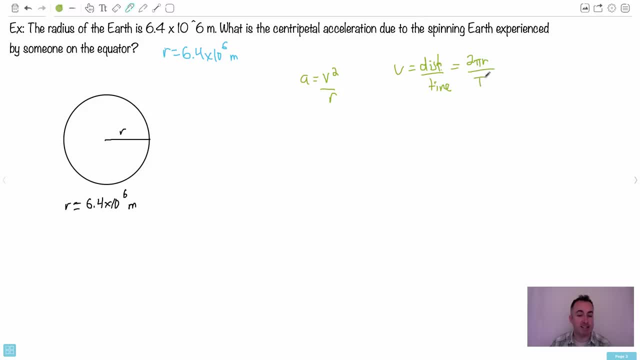 pi times R, All that divided by- usually we say T for the period of orbit. So in this case then it becomes V squared, which is 2 pi R over t. that's V, and then square that divided by R. It may not look that nice, so we can figure it out again. So E equals. let's see: 2 squared is 4 times pi squared. 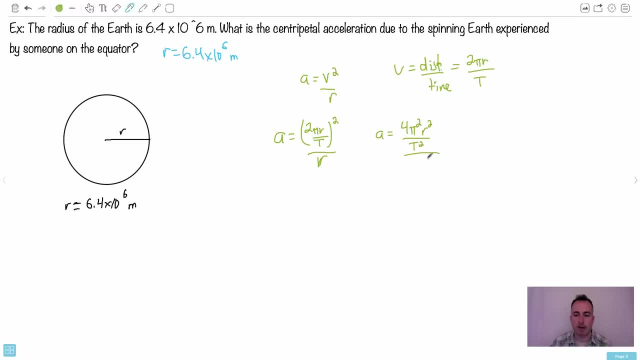 times R squared Times, R squared R. squared Times, R squared Times, R squared squared. I divide that whole thing by r. Now some people like to write this. I can write it as a fraction, just so you can see That means, when you divide by a fraction, what 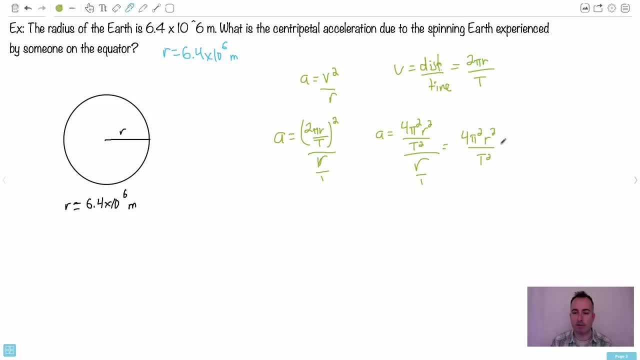 do you? do You multiply by the reciprocal? I'm just trying to make it more obvious to see what happens. Some people really struggle with this and putting the r on the bottom. That's just why it becomes like a one over r. You're going to see this r cancels out. 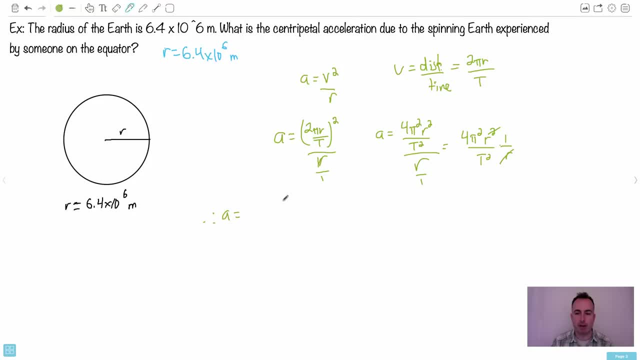 that one I'm left with acceleration is just equal to 4 pi squared r over t squared. Now this equation, this 4 pi squared r over t squared, turns out we've sort of re-derived an equation that's actually in your formula booklet. You didn't actually have to do all. 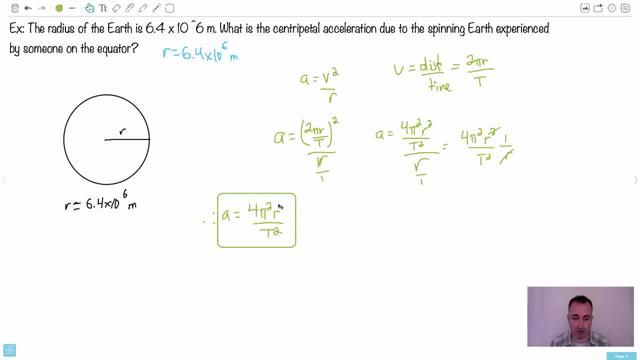 this work right here. that I did. You could have just looked this up and said, oh a, is 4 pi squared, r over t squared? Fine, Now remember, this is for someone who's sitting on earth, who's basically sitting on a planet. 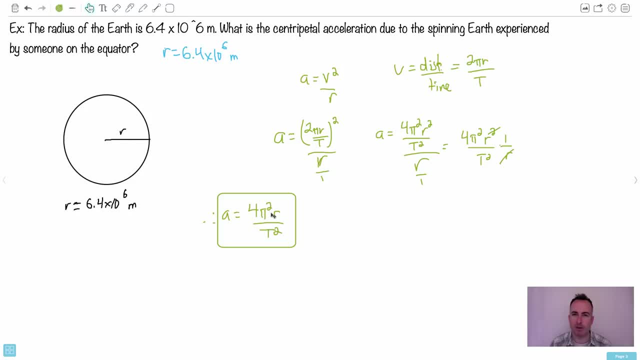 Basically rotating around the earth like this. What do we do now? Well, we need to know the period for someone on the earth. We need to know how long does it take to go all the way around the earth. You might know that number. Maybe we'll do this in a different. 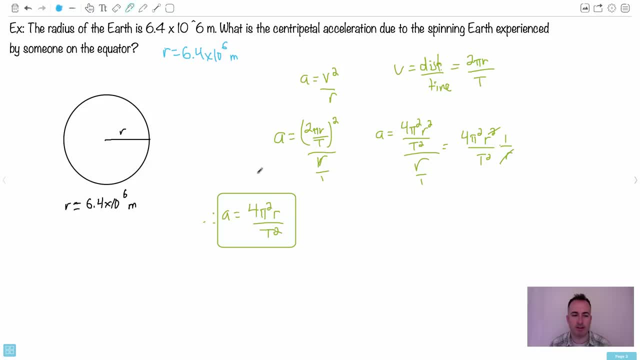 color here. Let's just figure this out here. How long does it take to go all the way around the earth? Do you know that value of t? I hope you do. It's 24 hours Now. we need this in seconds. What do we do? We use a trick that I learned in chemistry. 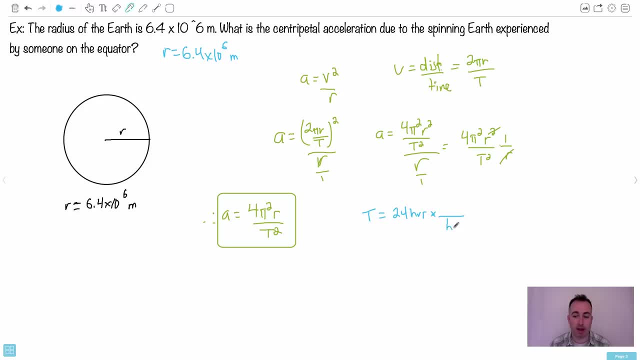 I just want to get rid of the hours. I'm going to put hours on the bottom. This way they're going to cancel out. I need to think about what will this do for me? I need to know something per hour In this case. I know there's 60 minutes in one hour. Now I know That's why. 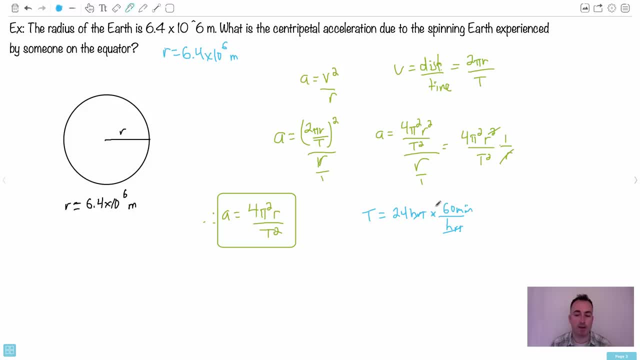 I put the minutes on top. There's 60 minutes for one hour. If I do 24 times 60, then I'm going to get my answer in minutes. I don't want it in minutes, I want it in seconds. You can use the same sort of trick here that the minutes are here You're going to have. 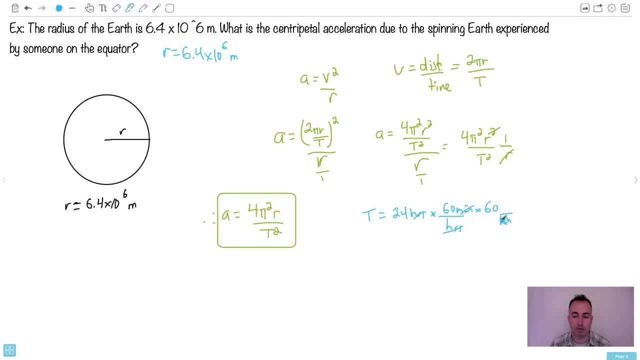 oops Minutes here The minutes will cancel out and then you'll have seconds. Then in the end, you're going to end up with this right here, which is 24 times 3600, which is 86400. 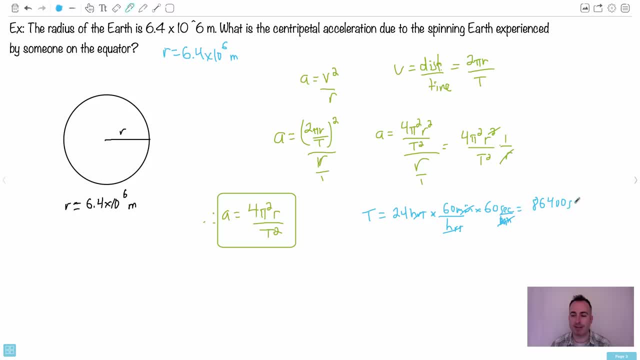 Technically, you should use a sidereal data, but good enough. This here is in seconds. This is my t. What I'm going to do now is put all this stuff into the equation. Finally, I have a equals 4.5.. 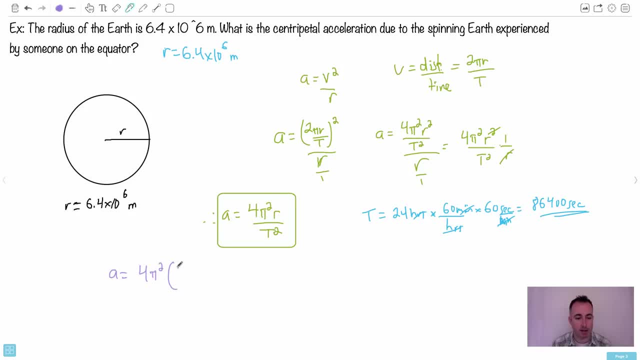 Pii squared times the radius, which is .4 times 10 to the sixth. all that divided by this number, It's 86400 seconds. That thing has to be squared. I'm going to get my answer. Let's see if we can figure it out. I'm just going to do that. so 6.4 times 10 to the sixth. 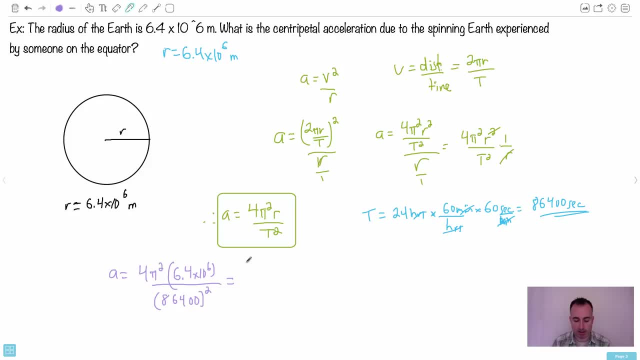 All that times, 4 times pi squared, I get that answer. divide that by, in brackets, 86400 squared, I end up with an acceleration of 0.0338, something like that. So how many significant figures can I use? Can I see? 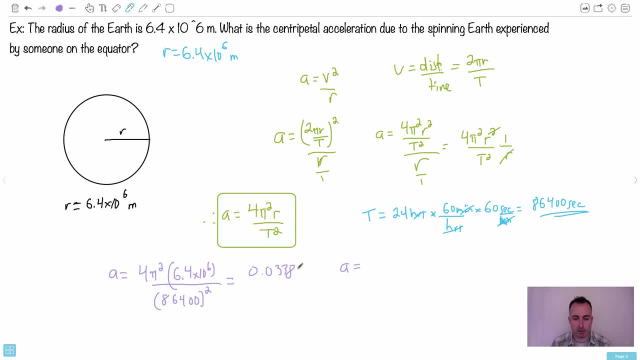 I use two. So I'm going to say, therefore, that my a equals, I guess, a zero point. I mean you could say just 0.03,, for example, meters per second squared. You can say: that's your answer. Think about this. this is very little compared to what we feel. 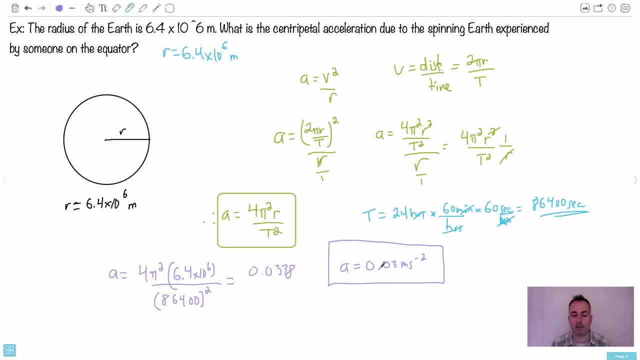 on Earth, right, I mean by gravity. So this is a yes, there's a slight acceleration inwards, but it's not very big, is it? We feel the acceleration due to gravity a lot more, But that's actually pretty interesting to figure. 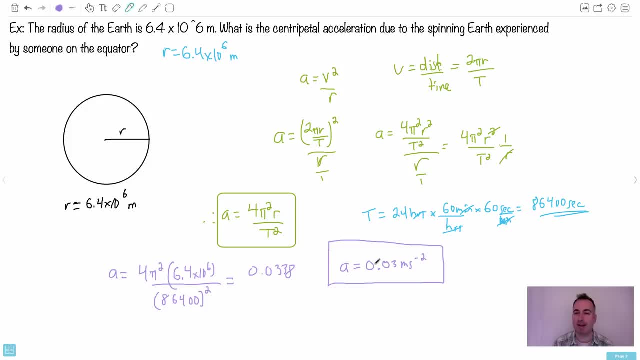 out what happens. So this is how we can deal with a question that might seem really hard but turns out we can solve it by just doing a little bit of algebra and a little bit of magic And, like I said, you can actually save a lot of time if 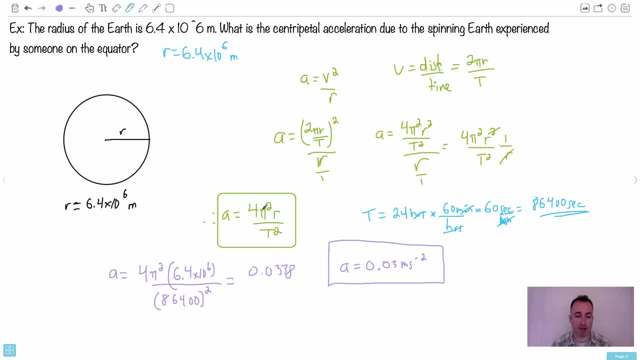 you're worried about this whole piece right here by just starting off right away with a equals 4 pi squared, r over t squared. You just have to know the picture Period, How long it takes to go around the Earth.